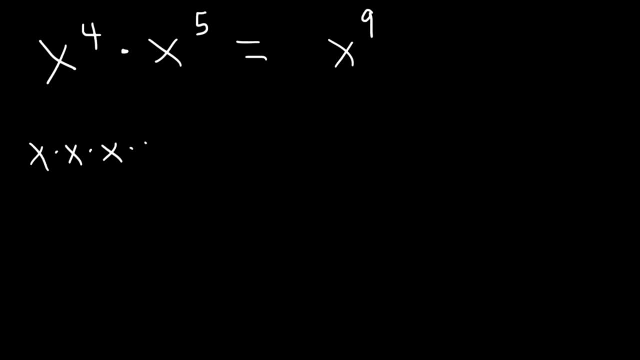 x to the 4th is basically multiplying 4x variables together, And x to the 5th is equivalent to multiplying 5x variables together, So in total you're multiplying 9x variables together, And so that's why it's equal to x to the 9th. 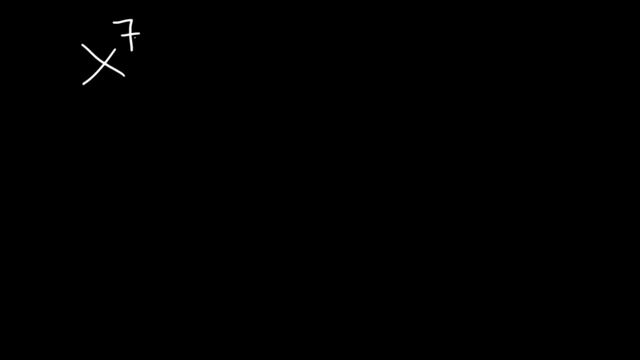 Now what about division? Let's say, if you divide by a common base, What should you do with the exponents? You need to subtract x to the 7th, Divided by x to the 3th. we need to subtract 7 by 3.. 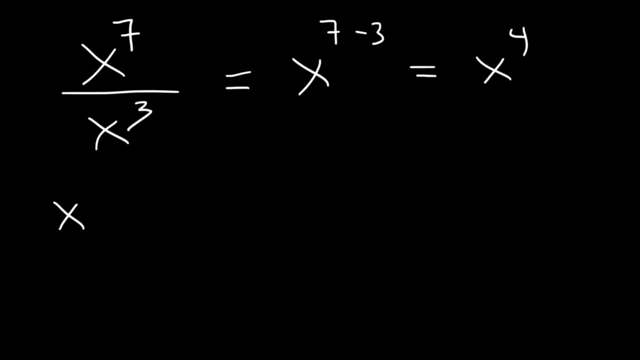 And that's going to be x to the 4th. x to the 7th is equivalent to 7x variables multiplied to each other, And x cubed is simply x times x times x. So we can cancel 3x variables which leave behind 4x variables on top. 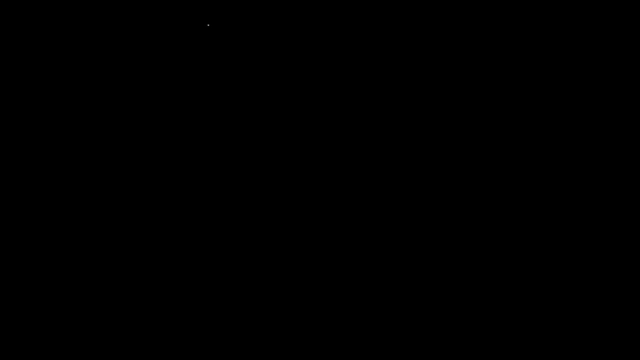 And so that's the answer. Here's another one. What is x to the 3rd, Raised to the 4th power? What should we do whenever we raise one exponent to another? In a situation like this, you need to multiply. 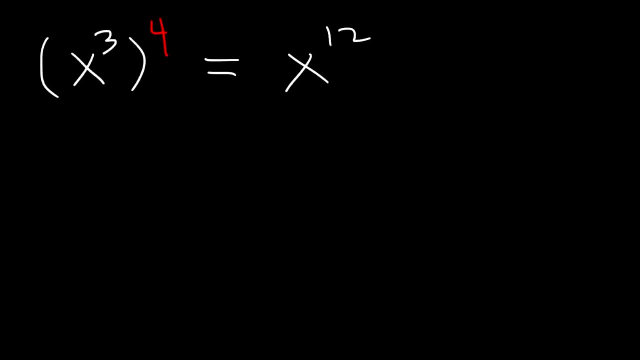 It's going to be 3 times 4, which is 12.. So x to the 3rd, raised to the 4th, power means that you're multiplying 4x cubed values, And each x cubed is basically 3x variables multiplied to each other. 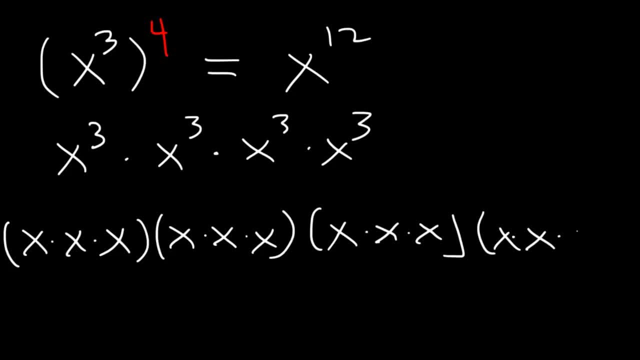 So if you count all the x variables, what we have is a total of 12.. And so that's why it's equal to x to the 12th. Now, what about x raised to the 0 power? What is that equal to? 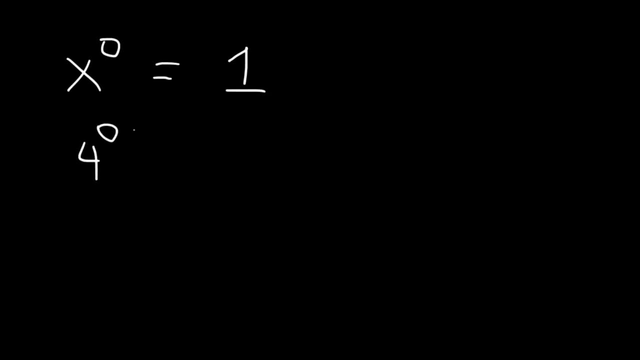 Anything raised to the 0, power is 1.. So 4 to the 0 is 1.. Now what about x raised to the negative 3?? What should we do if we have negative exponents? If you have a negative exponent, all you could do is take the variable, move it to the bottom. 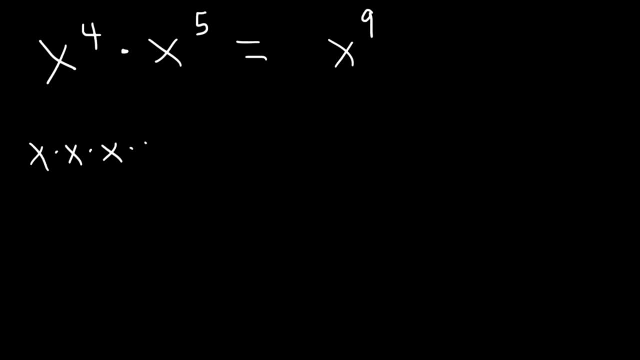 x to the 4th is basically multiplying 4x variables together, And x to the 5th is equivalent to multiplying 5x variables together, So in total you're multiplying 9x variables together, And so that's why it's equal to x to the 9th. 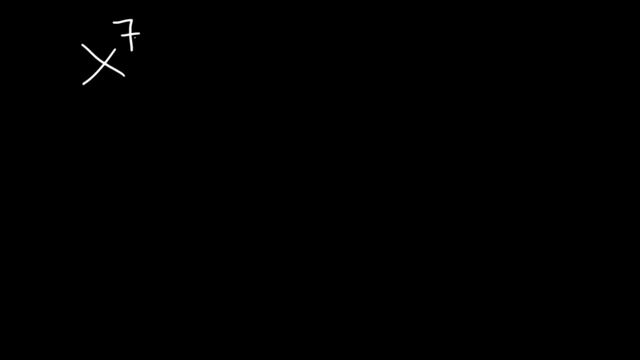 Now what about division? Let's say, if you divide by a common base, What should you do with the exponents? You need to subtract x to the 7th, Divided by x to the 3th. we need to subtract 7 by 3.. 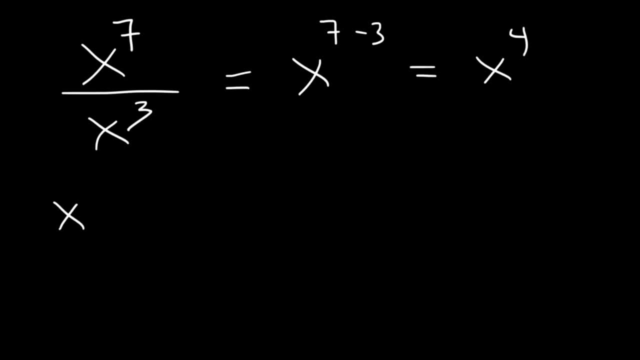 And that's going to be x to the 4th. x to the 7th is equivalent to 7x variables multiplied to each other, And x cubed is simply x times x times x. So we can cancel 3x variables which leave behind 4x variables on top. 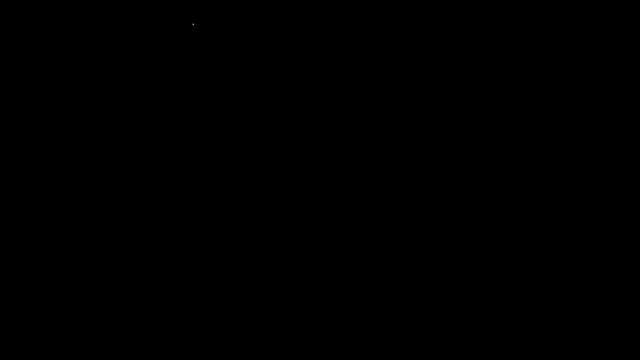 And so that's the answer. Here's another one. What is x to the 3rd, Raised to the 4th power? What should we do whenever we raise one exponent to another? In a situation like this, you need to multiply. 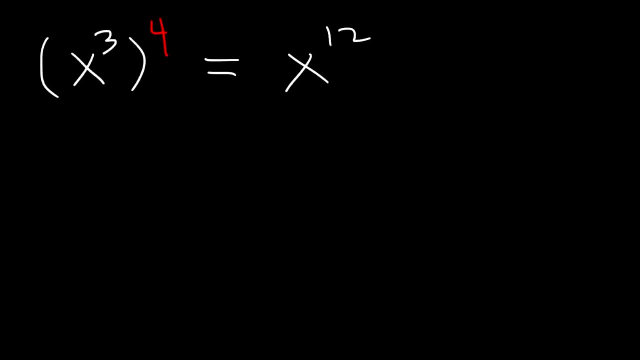 It's going to be 3 times 4, which is 12.. So x to the 3rd, raised to the 4th, power means that you're multiplying 4x cubed values, And each x cubed is basically 3x variables multiplied to each other. 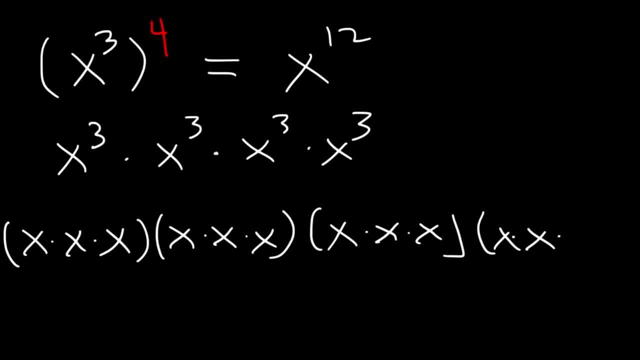 So if you count all the x variables, what we have is a total of 12.. And so that's why it's equal to x to the 12th. Now, what about x raised to the 0 power? What is that equal to? 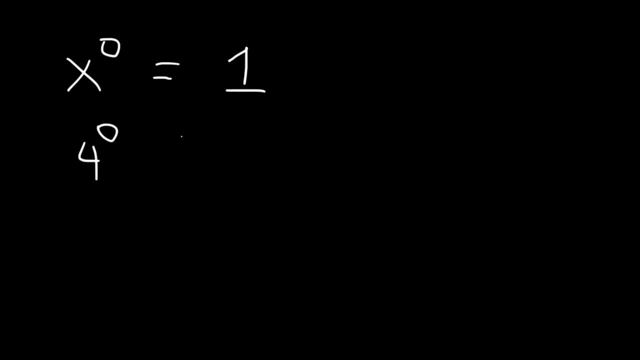 Anything raised to the 0, power is 1.. So 4 to the 0 is 1.. Now what about x raised to the negative 3?? What should we do if we have negative x? What should we do if we have negative exponents? 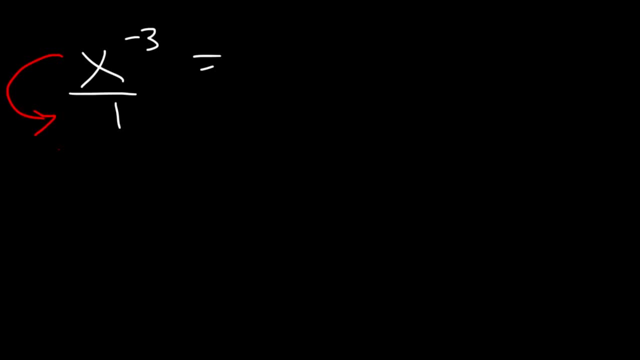 If you have a negative exponent, all you could do is take the variable and move it to the bottom. When you do that, the negative 3 will become positive 3. And so it's 1 over x cubed. Likewise, let's say, if you have 1 divided by x, raised to the negative 4.. 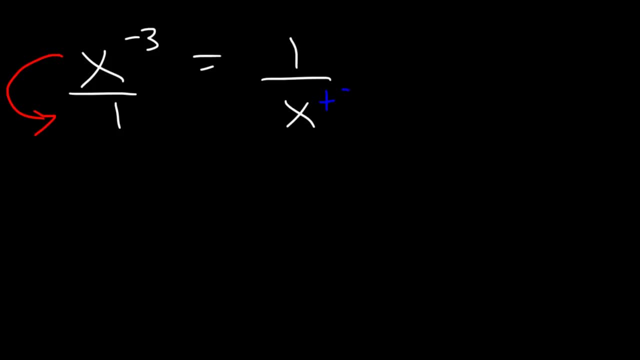 When you do that, the negative 3 will become positive 3. And so it's 1 over x cubed. Likewise, let's say, if you have 1 divided by x raised to the negative 4. You can move the x variable to the top and the exponent will change sign. 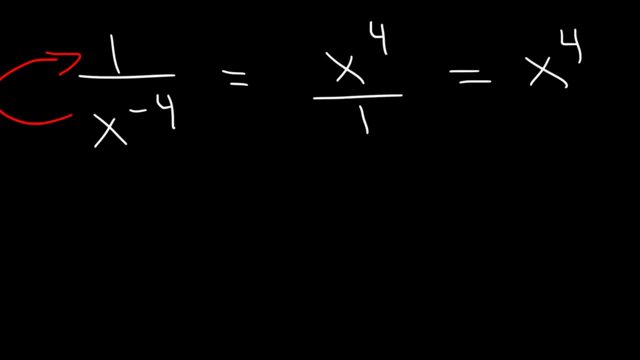 So it's going to be x to the positive, 4 over 1.. Or simply x raised to the 4th power. Now here's a question for you: What is the value of negative 3 squared? What do you think that's equal to? 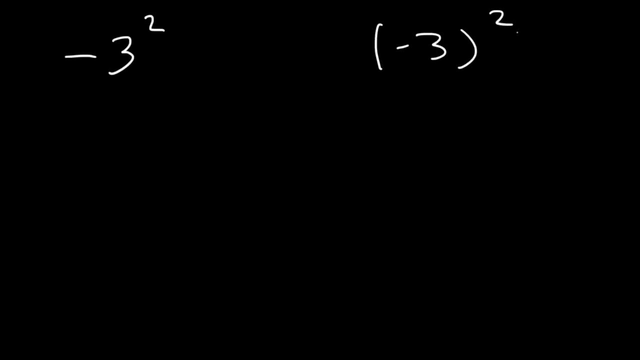 Now what about negative 3 squared within the parentheses? Negative 3 squared is basically negative 3 times negative 3.. We have two of them, So this is equal to positive 9.. Now what we have here is one negative and two 3's. 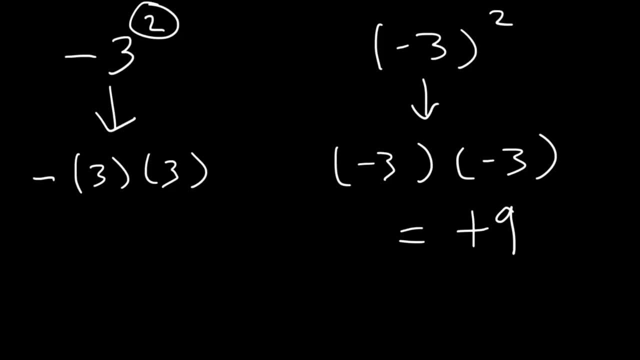 This 2 does not apply to the negative sign, so we only have one negative sign. So this is negative. and then 3 times 3 is 9, so the whole answer is negative 9.. So just keep in mind the difference between the two. 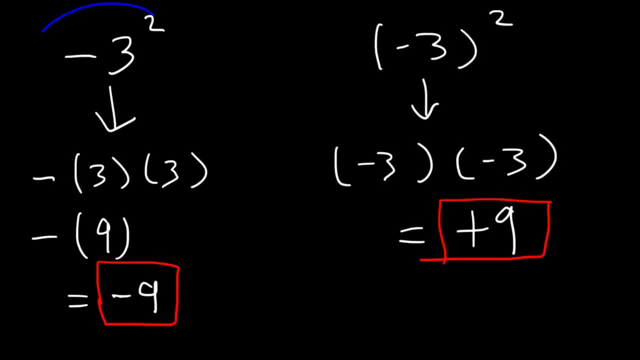 You can confirm this in the calculator. If you type in negative 3 squared- just the way you see it like this- you should get negative 9.. But if you type it like this in your calculator, it should give you positive 9.. 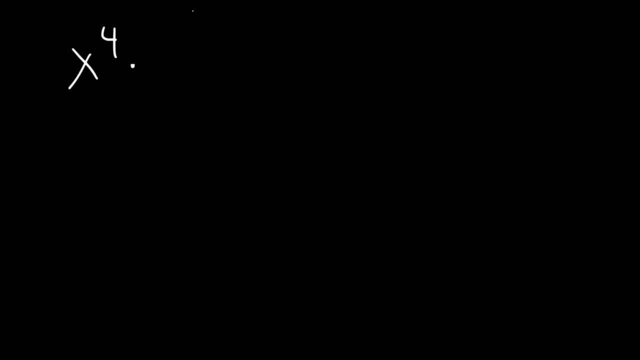 Go ahead and simplify these problems. Simplify the following expressions: 1. This is the first one, So here's the first one: X cubed raised to the negative. 5. Also, x to the seventh power divided by x to the twelfth. 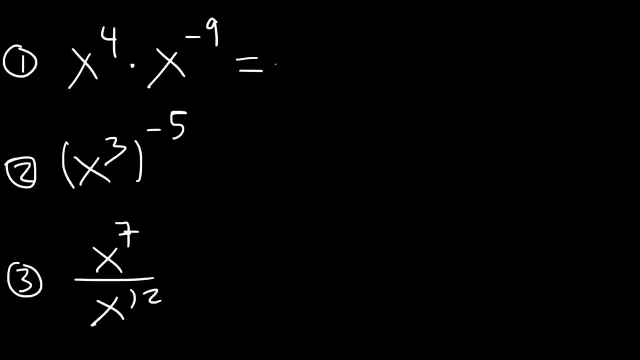 Go ahead and work on these examples. So when multiplying common bases you need to add the exponents 4 plus negative. 9 is negative five. X raised to the negative 5 is equivalent to 1 over x to the fifth. So if I get any negative exponents, 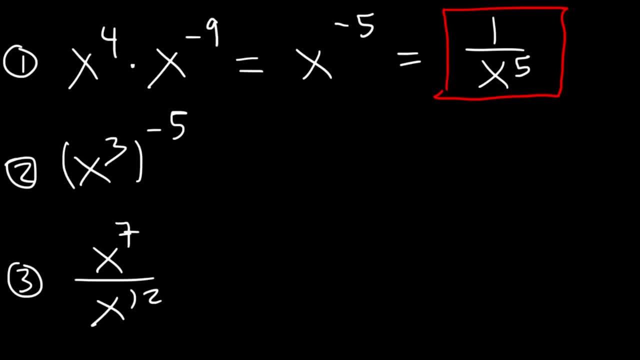 Other things that you can do is you can add the exponents, make it positive. now here we have one exponent raised to another, so we need to multiply 3 times negative 5 is negative 15. X to the negative 15 is 1 over X to. 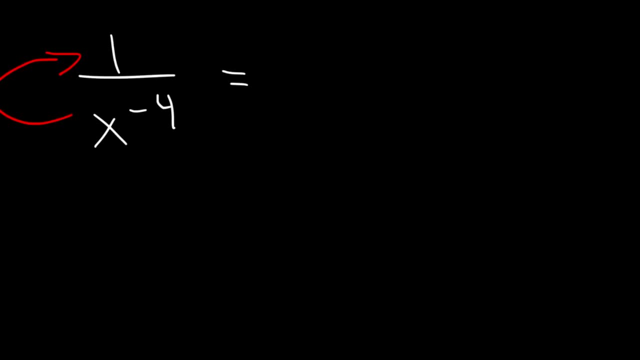 You can move the x variable to the top and the exponent will change sign. So it's going to be x to the positive, 4 over 1, or simply x raised to the 4th power. Now here's a question: What is the value of negative 3 squared? 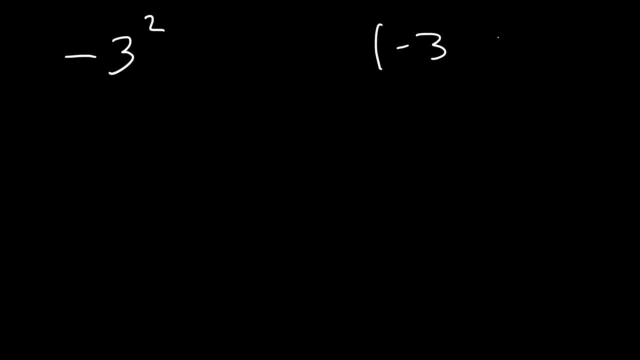 What do you think that's equal to? Now what about negative 3 squared? within a parenthesis? Negative 3 squared is basically negative 3 times negative 3.. We have two of them, So this is equal to positive 9.. Now what we have here is one negative and two 3s. 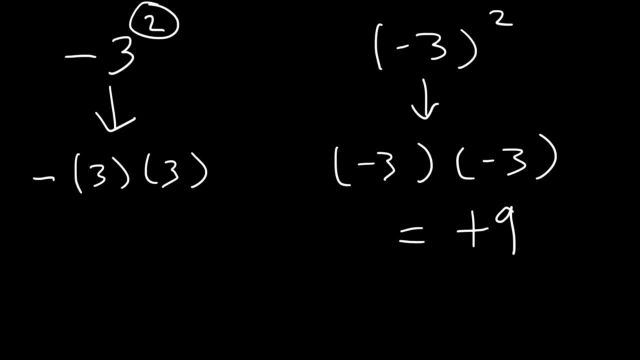 This 2 does not apply to the negative sign, so we only have one negative sign. So this is negative. And then 3 times 3 is 9, so the whole answer is negative 9.. So just keep in mind the difference between the two. 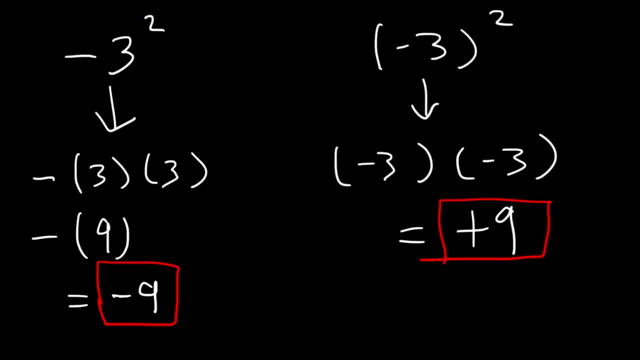 You can confirm this in the calculator. If you type in negative 3 squared- just the way you see it like this- you should get negative 9.. But if you type it like this in your calculator, it should give you positive 9.. 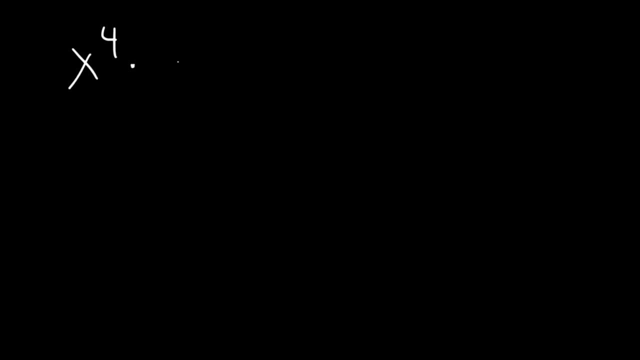 Go ahead and simplify these problems, Simplify the following expressions. So let's say this is the first one. Here's the next one: x cubed raised to the negative, 5.. And also x to the 7th, power divided by x to the 12th. 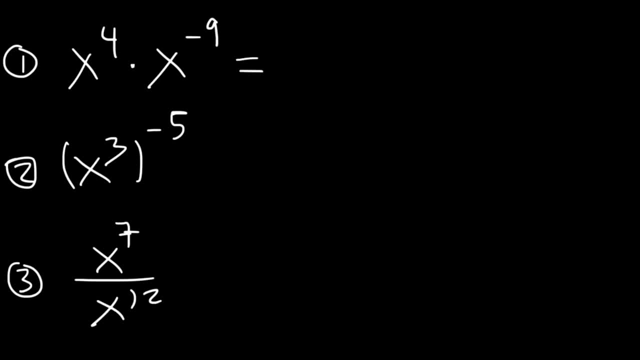 Go ahead and work on these examples. So when multiplying common bases, you need to add the exponents 4 plus negative 9 is negative 5.. And x raised to the negative 5 is equivalent to 1 over x to the 5th. 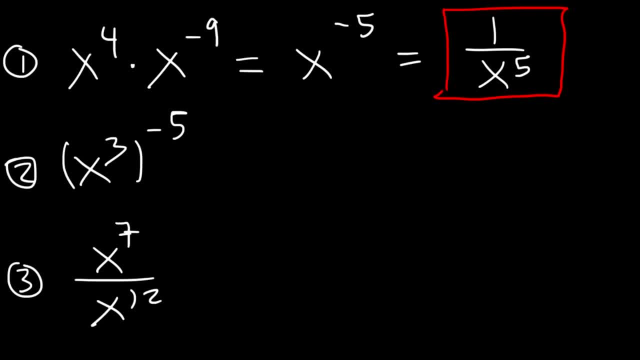 So if you get any negative exponents, make it positive. Now here we have one exponent raised to another, So we need to multiply 3 times negative, 5 is negative, 15.. x to the negative 15 is 1 over x to the positive 15.. 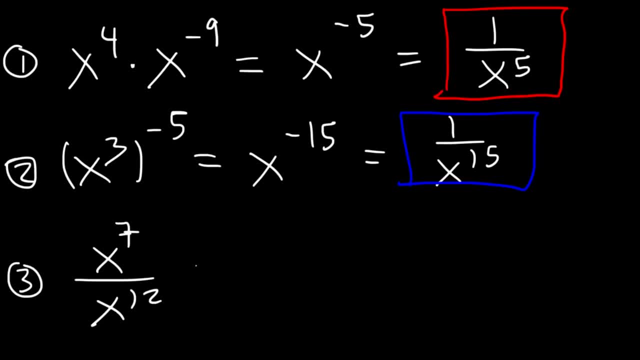 So this is the final answer for that problem. Now for the last one. we need to subtract. We need to take the top number and subtract it by the bottom number. 7 minus 12 is negative 5. And this is the same as 1 over x. 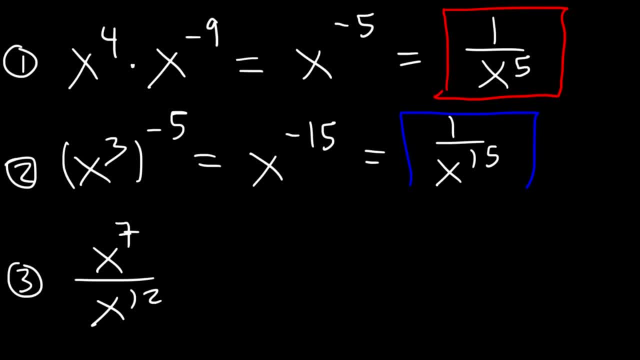 the positive 15. so this is the final answer for that problem. now for the last one. we need to subtract. we need to take the top number and subtract it by the bottom number. 7 minus 12 is negative 5 and this is the same as 1 over X to the. 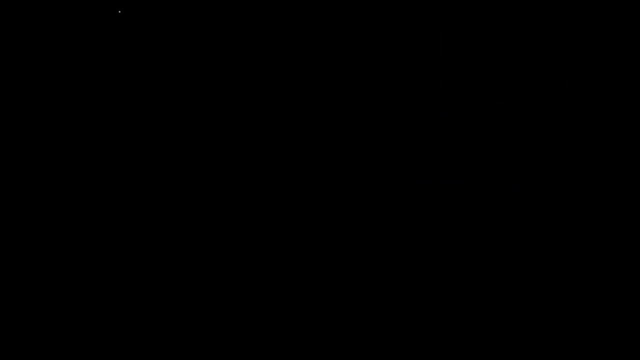 5. now let's talk about that example. X to 7 means that we have 7 X variables. X to 12 means that we have a total of 12 X variables multiplied to each other. so we can cancel all seven X variables on top and seven on the bottom and 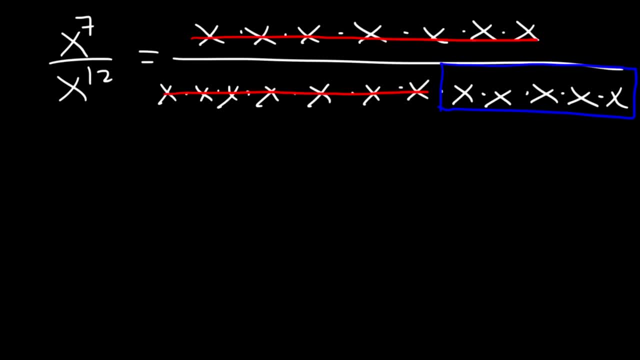 notice that we have five X variables left on the bottom, and that's why it's 1 over X to the 5. what is the value of 3x squared raised to the third power? go ahead and simplify this expression, so 3 is the same as 3 to the first whenever you raise one exponent to 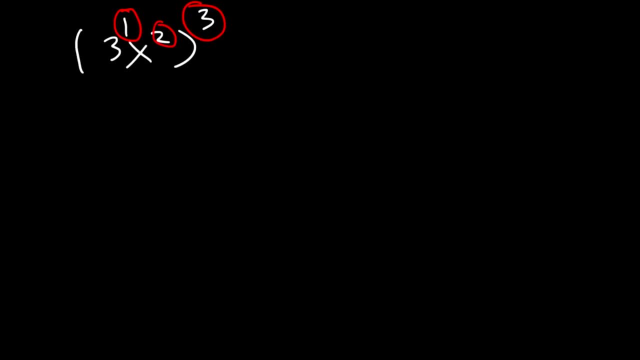 another. you need to multiply, but we have two exponents here, so we need to distribute the 3 to the 1 and to the 2. so 3 times 1 is 3 and 2 times 3 is 6. so this is 3 to the third, times X to the 6. so what's? 3 to the third, 3 to the third. 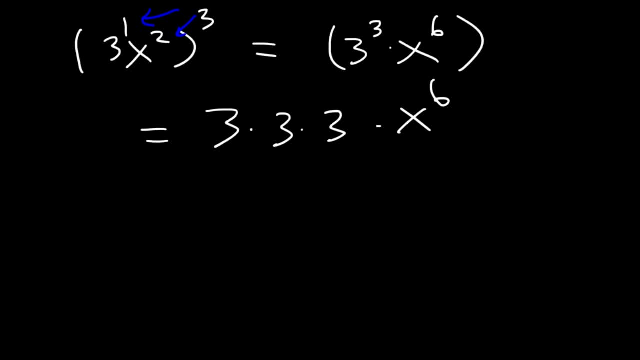 is 3 times 3 times 3, 3 times 3 is 9 and 9 times 3 is 27. so the final answer is 27 times X, raised to 6 power. try this one negative 2. ok, that doesn't look like a 2, let's do that. 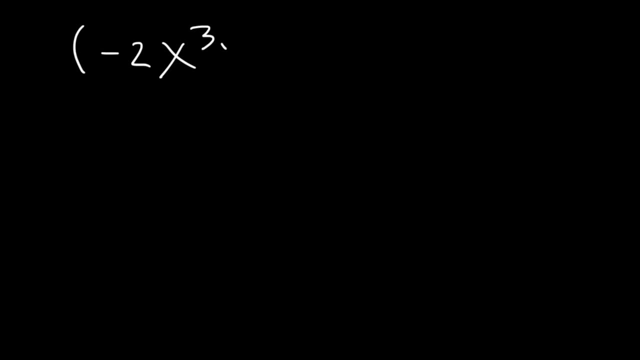 again negative 2x cubed Y to the fourth, raised to the second power. feel free to pause the video and work on that example. so this is raised to the first power and if we multiply by two we're going to have negative 2 to the second power. and then three times 2 is 6, so we're going. 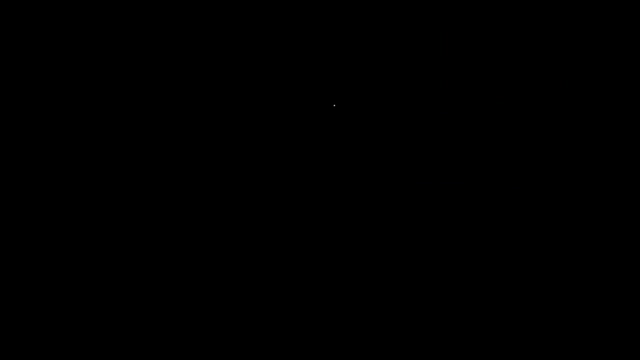 x to the 5.. Now let's talk about that example. x to the 7th means that we have 7 x variables. x to the 12th means that we have a total of 12 x variables multiplied to each other. 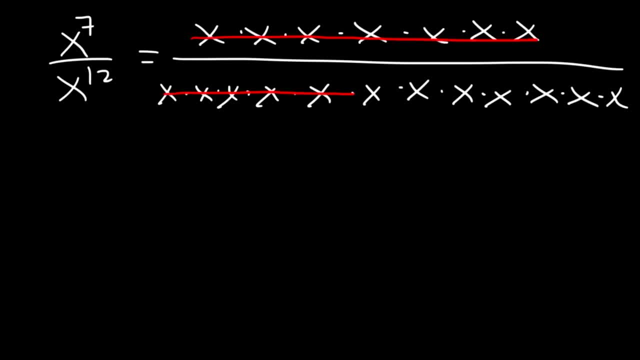 So we can cancel all 7 x variables on top and 7 on the bottom And notice that we have five x-verbals left on the bottom and that's why it's 1 over x to the 5.. What is the value of 3x squared raised to the third power? 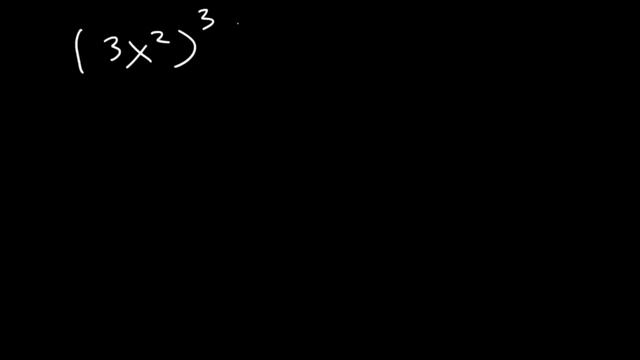 Go ahead and simplify this expression. So 3 is the same as 3 to the first. Whenever you raise one exponent to another, you need to multiply, But we have two exponents here, so we need to distribute the 3 to the 1 and. 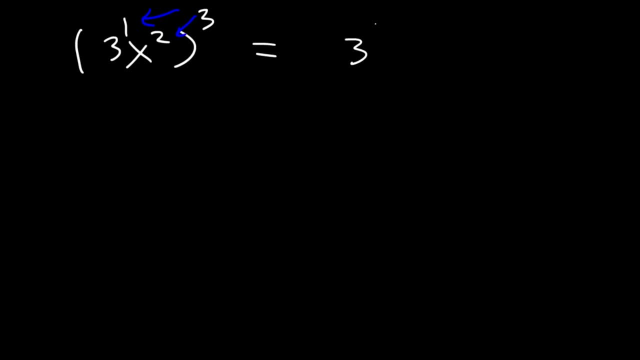 to the 2.. So 3 times 1 is 3, and 2 times 3 is 6.. So this is 3 to the third times x to the 6.. So what's 3 to the third? 3 to the third is 3 times 3 times 3.. 3 times 3 is 9,. 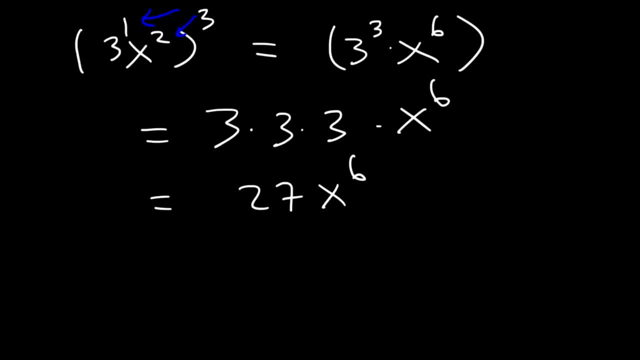 and 9 times 3 is 27.. So the final answer is 27.. So this is 3 to the third times x raised to the sixth power. Try this one: Negative: 2.. Okay, that doesn't look like a 2. Let's do that again. Negative. 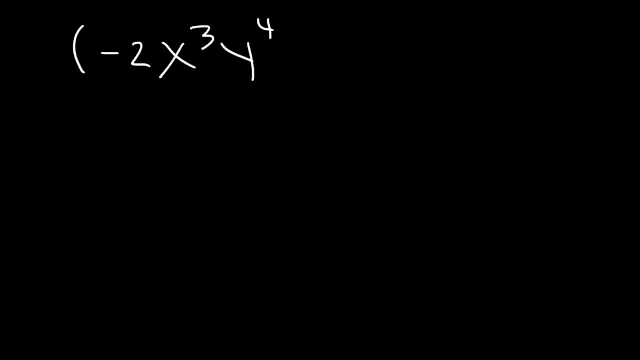 2 x cubed y to the fourth, raised to the second power. Feel free to pause the video and work on that example. So this is raised to the first power and if we multiply it by 2, we're going to have negative 2 to the second power. 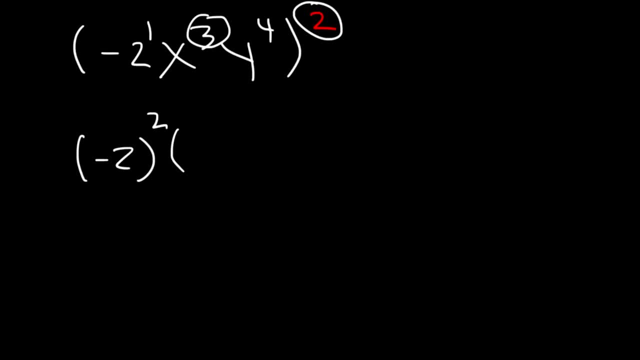 And then 3 times 2 is 6.. So we're going to have x to the sixth And 4 times 2 is 8.. So this is going to be y to the eighth. Negative 2 squared, that's basically negative 2 times. 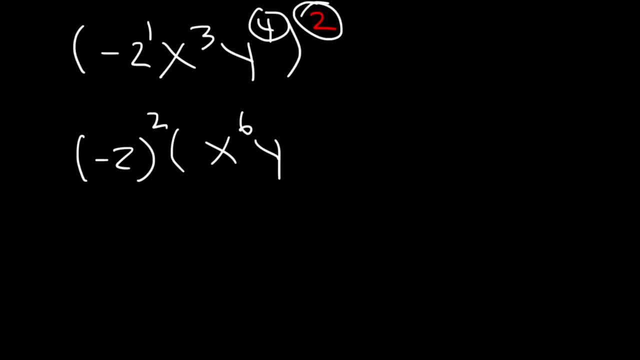 to have X to the sixth, and 4 times 2 is 8. so this is going to be Y to the 8. negative 2 squared, that's basically negative 2 times negative 2. that's equal to positive 4. so the answer is for X to the 6. 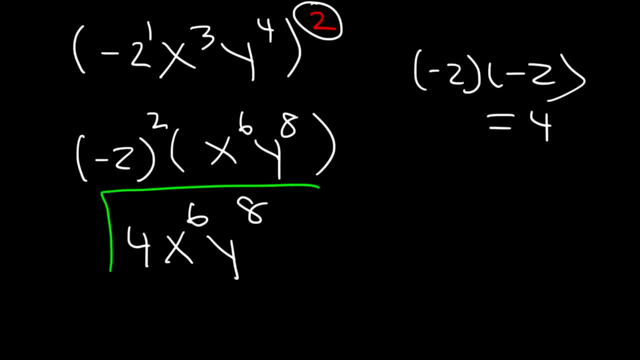 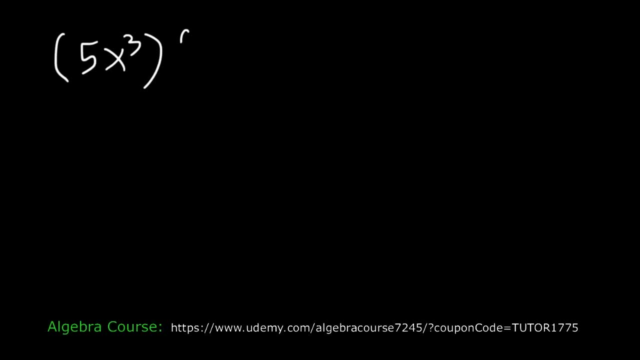 Y raised to the fourth to the eighth power, What is the value of 5x cubed multiplied by 4x to the seventh power? So what should we do in this example? So first we need to multiply 5 times 4.. 5 times 4 is 20, and then we need to multiply x cubed times x to the 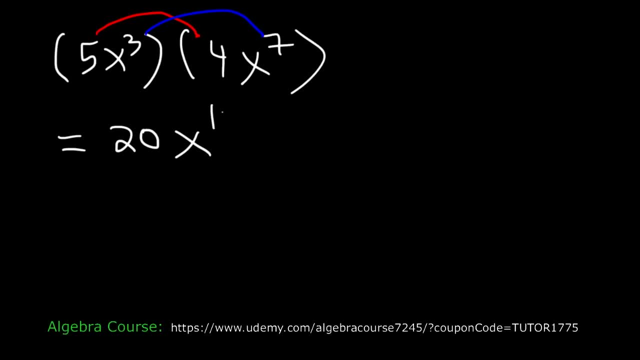 seventh, in which case we need to add: 3 plus 7 is 10, so this is simply 20 x to the tenth. So try this example: 7x to the sixth times, 5x to the fourth and also 4x. 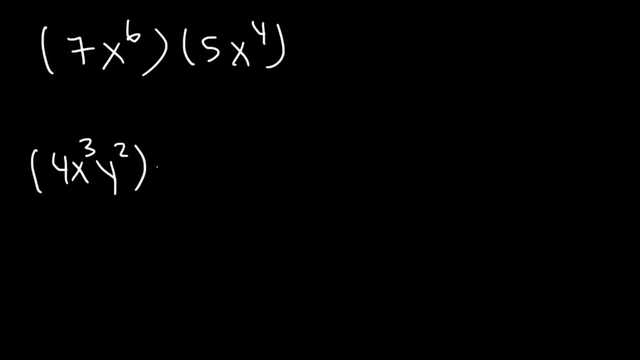 cubed y squared times 7x to the negative fourth, y to the third. So in the first example we need to multiply 7 by 5.. 7 times 5 is 35. and then we get to multiply x to the sixth times x to the fourth. 6 plus 4 is 10, so it's 35 x to the tenth. 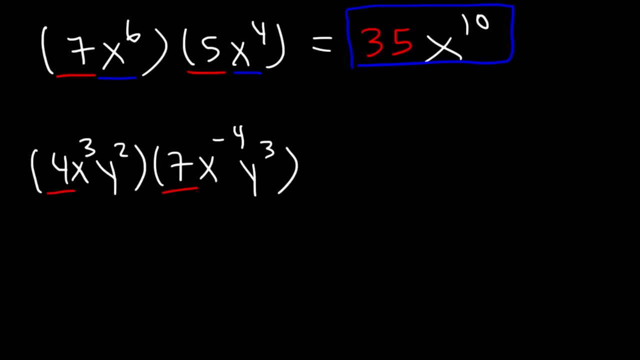 Now the next example: we're going to multiply 4 by 7, which is 28, and then x cubed times x to the negative fourth. So we're going to add 3 plus negative 4, which is negative 1, and then, finally, we're going to multiply y squared times y cubed. 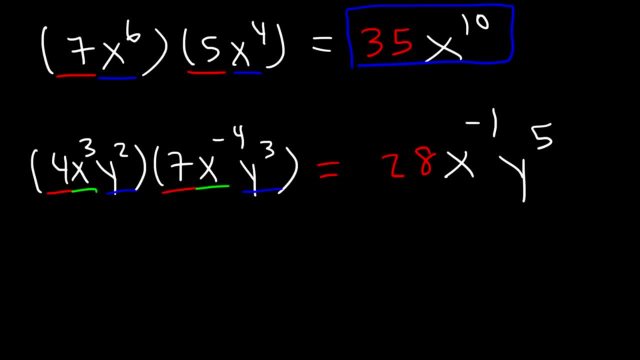 2 plus 3 is 5, so it's y to the fifth power. Now we need to get rid of the negative exponent, So let's move the x variable to the bottom. So it's 28 y to the fifth divided by x, and so that's the answer. 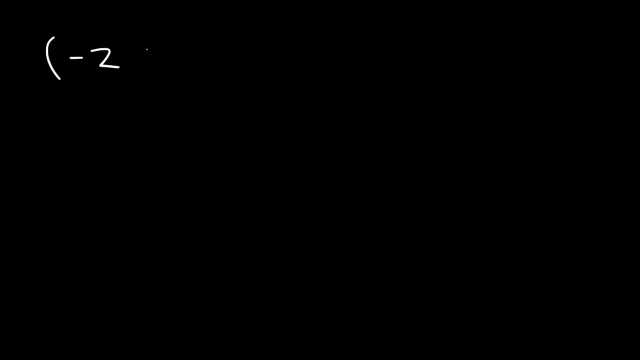 What is negative 2x cubed y raised to the zero power? What is that equal to? Anything raised to the zero power. keep in mind it's 1.. Now, what about negative 4x to the zero power? What is that equal to? You need to realize that. 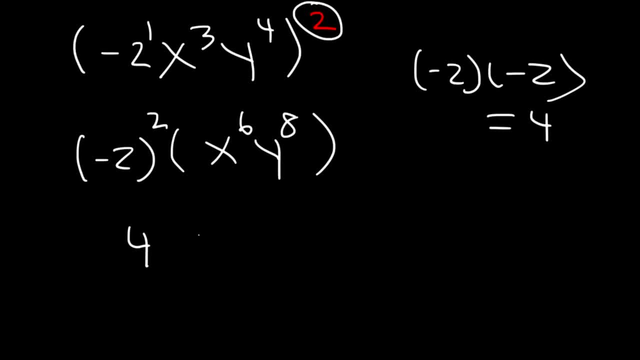 negative 2. That's equal to positive 4.. So the answer is 4 x to the sixth, y raised to the eighth power. What is the value of 5x cubed multiplied by 4x to the seventh power? So what should we do in this example? So first we need to multiply 5 times 4.. 5 times 4 is 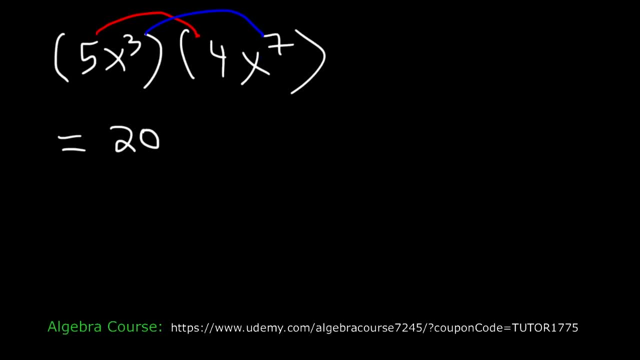 20.. And then we need to multiply x cubed times x to the seventh, in which case we need to add: 3 plus 7 is 10.. So this is simply 20 x to the tenth. So try this example: 7 x to. 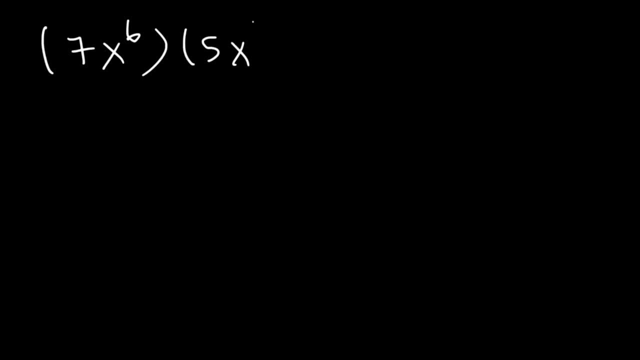 the sixth times 5x to the fourth. So 3 plus 7 is 10.. So this is simply 20 x to the tenth. Try this example: 7, x to the x to the 4th, and also 4x cubed y squared times 7, x to the negative 4th, y to the 3rd. 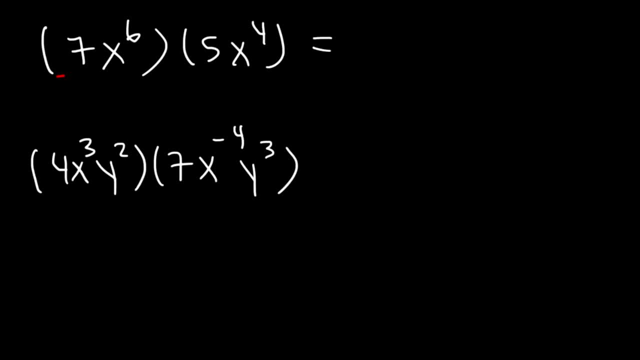 So in the first example we need to multiply 7 by 5.. 7 times 5 is 35, and then we got to multiply x to the 6th times x to the 4th. 6 plus 4 is 10, so it's 35x to the 10.. 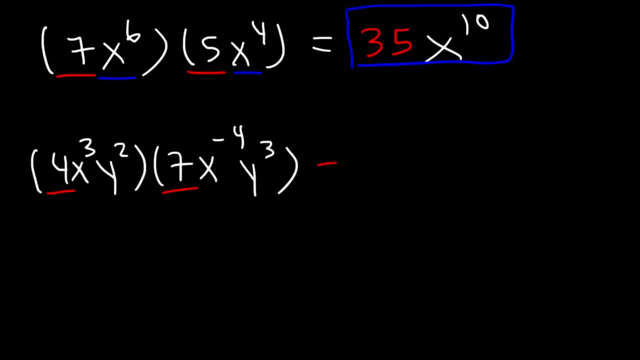 Now in the next example, we got to multiply 4 by 7,, which is 28,, and then x cubed times x to the negative 4th, so we got to add 3 plus negative 4,, which is a negative 1, and 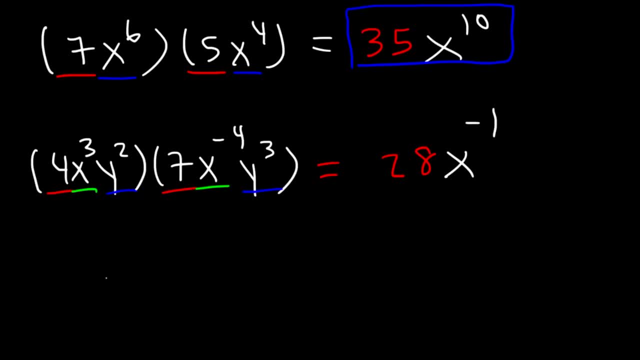 then, finally, we got to multiply y squared times, y cubed 2 plus 3 is 5, so it's y to the 5th power. Now we need to get rid of the negative exponent, so let's move the x variable to the bottom. 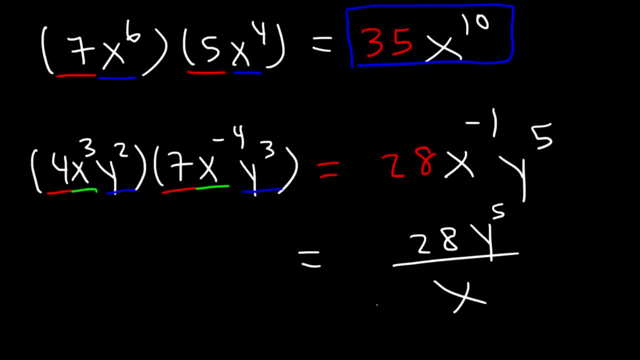 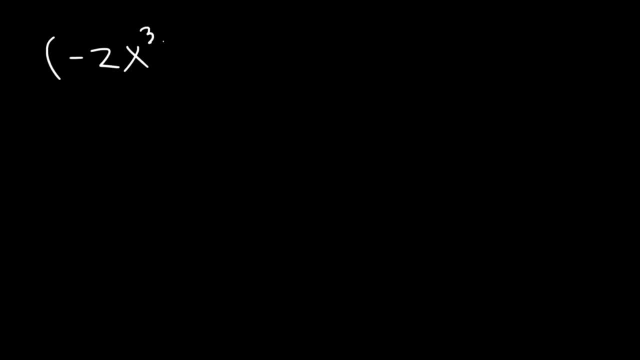 So it's 28y to the 5th Divided by x. and so that's the answer. What is negative? 2x cubed y raised to the 0th power, What is that? equal to Anything raised to the 0th power. keep in mind it's 1.. 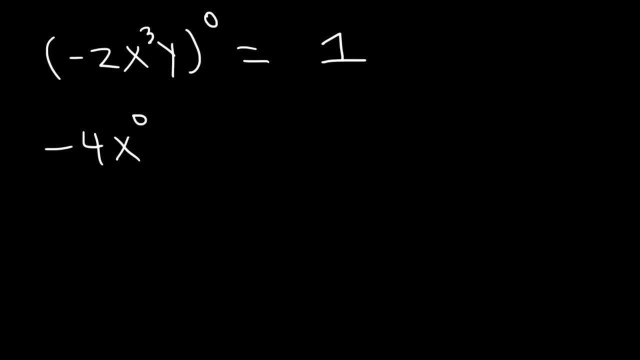 Now, what about negative 4x to the 0th power? What is that equal to? You need to realize that this is negative 4 times x raised to the 0th power. The 0 only applies to x, So this portion. 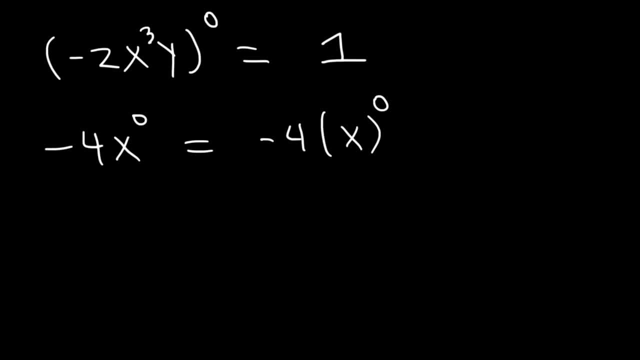 this is negative 4 times x. raised to the zero power, The zero only applies to x. So this portion highlighted in red, that's equal to 1.. So it's negative 4 times 1 and that's negative 4.. So anything that's affected by the zero exponent will. 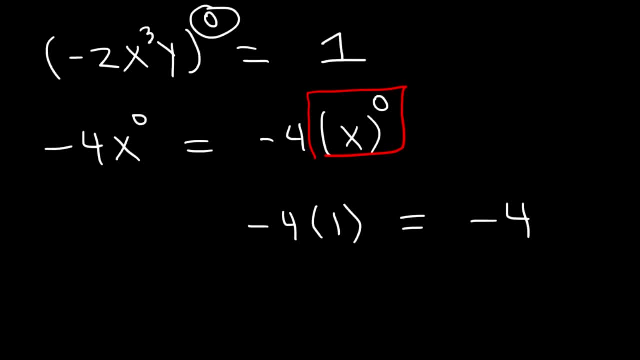 become a 1.. Anything outside of that is unaffected. Try this problem: What is 24x to the 7th, y to the 3rd, divided by 8x to the 4th, y to the negative 12?? So in this case we need to divide 24. divided by 8 is 3.. x to the 7th. 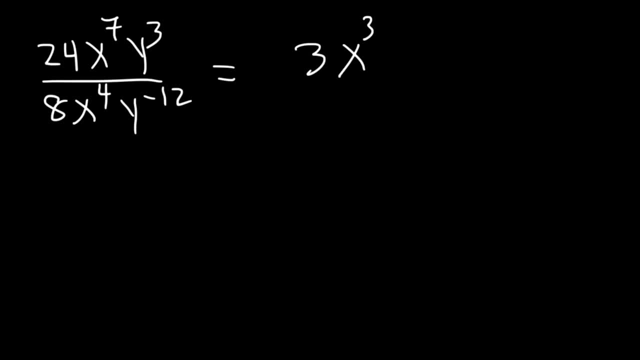 divided by x to the 4th is x. cubed, 7 minus 4 is 3.. And for the y variables we need to subtract: 3 minus negative. 12 is the same as 3 plus 12.. So this becomes y. 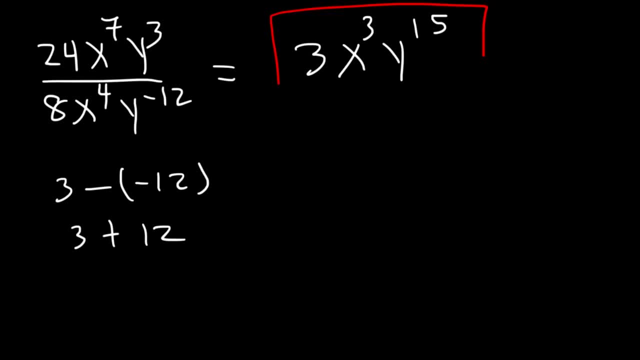 to the 15th, And so that's the answer. What is 35x, cubed y to the 5th, divided by 63x to the negative, 4th, y to the 7th, squared, What is that equal to? 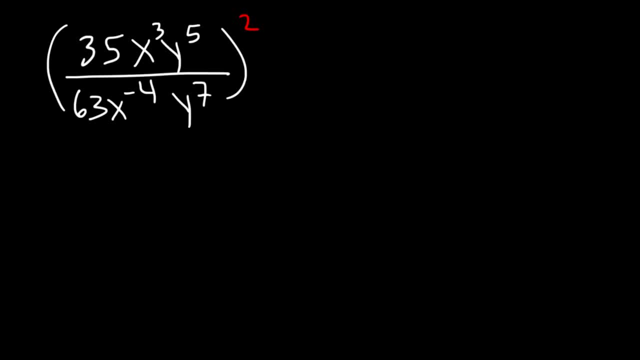 So we could distribute the two or we could simplify first, We could divide first or distribute the exponent. Let's divide first. 35 is basically 5 times 7, and 63 is 9 times 7.. Now x to the 3rd divided by x to the negative, 4.. 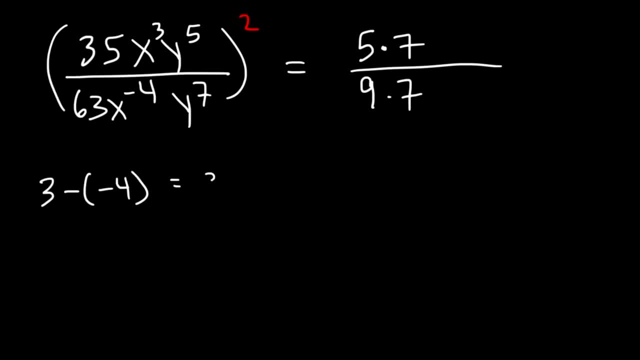 That's going to be 3 minus negative 4, which is 3 plus 4, and that's 7.. So we're going to have x to the 7th on top, And then we have 5 minus 7, which is negative 2. It's. 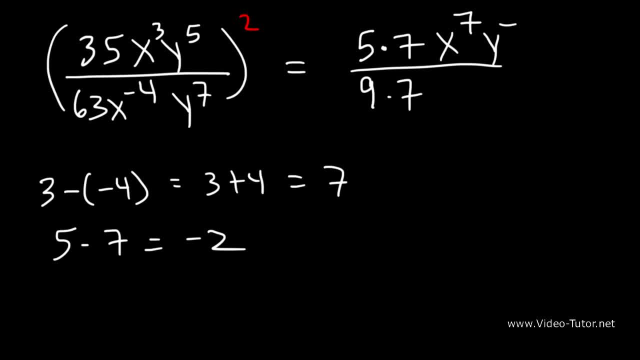 negative 2 on top, but if we bring it to the bottom it's going to be positive 2 on the bottom. So let's go ahead and do that. And this is still raised to the second power. Now the last thing we could do is cancel. 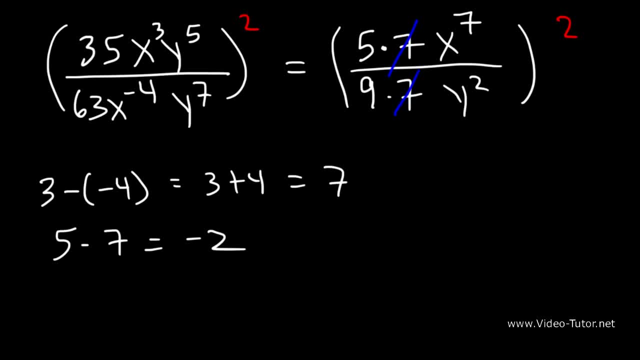 the 7.. Let's get rid of this stuff. So we have 5 x to the 7th divided by 9 y squared raised to the second power, 5 squared is 25 and x to the 7th raised to the second. 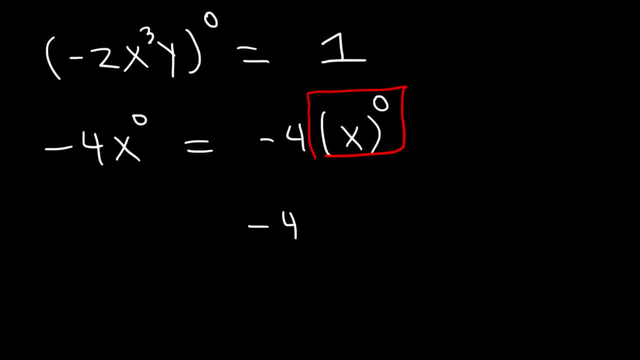 Highlighted in red, that's equal to 1.. So it's negative 4 times 1, and that's negative 4.. So anything that's affected by the 0 exponent will become a 1.. Anything outside of that is unaffected. 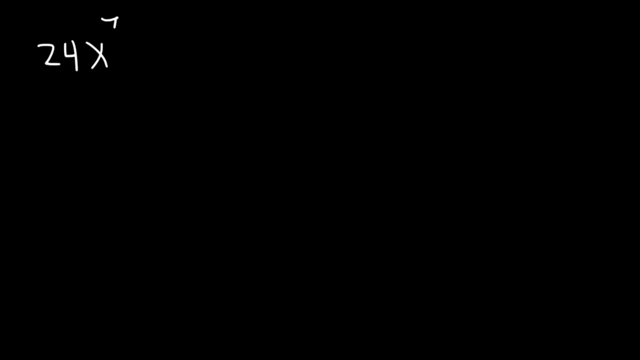 Try this problem: What is 24x to the 7th y to the 3rd, divided by 8x to the 4th, y to the negative 12th? So in this case we need to divide 24 divided. 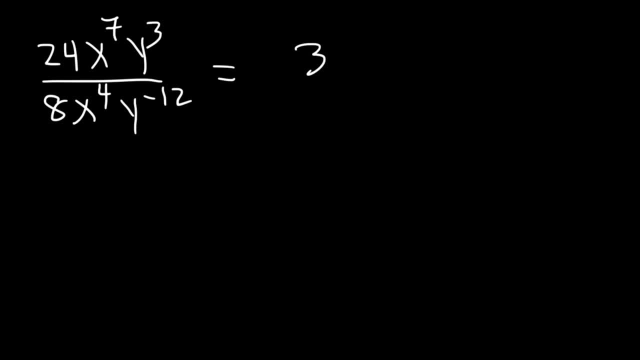 divided by 8 is 3.. x to the 7th divided by x to the 4th is x. cubed, 7 minus 4 is 3.. And for the y variables we need to subtract: 3 minus negative 12 is the same as 3 plus 12.. 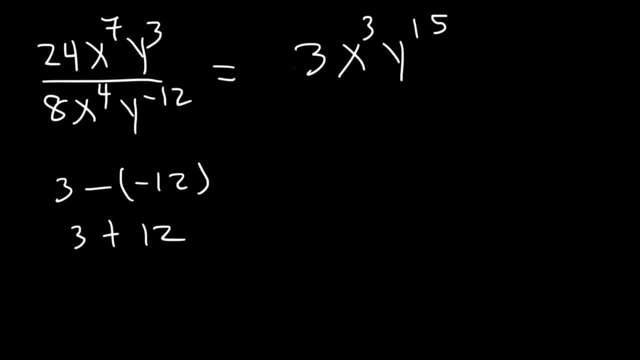 So this becomes y to the 15th, And so that's the answer. What is 35x cubed, y to the 5th divided by 63?? x to the negative 4th, y to the 7th squared, What is that equal to? 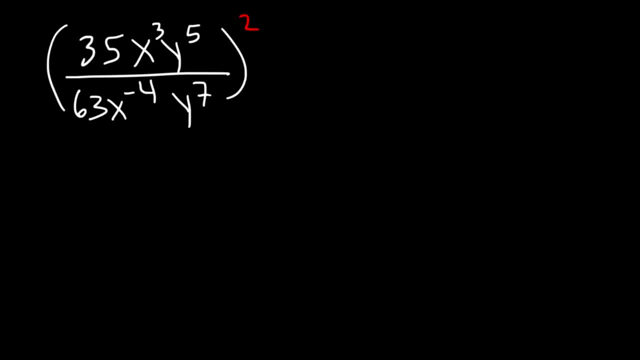 So we could distribute the 2, or we could simplify first, We could divide first or distribute the exponent. Let's divide first. 35 is basically 5 times 7.. And 63 is 9 times 7.. Now x to the 3rd divided by: 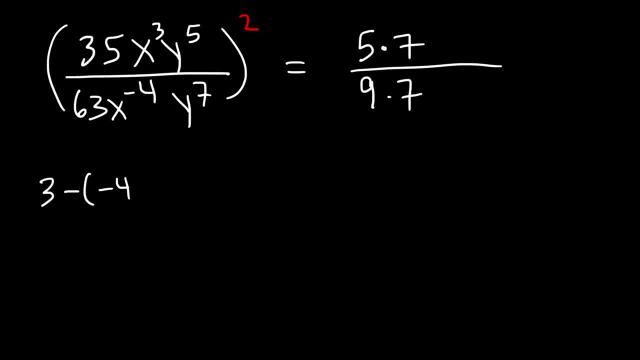 x to the negative 4th, That's going to be 3 minus negative 4, which is 3 plus 4, and that's 7.. So we're going to have x to the 7th on top, And then we have 5 minus 7, which is negative 2.. 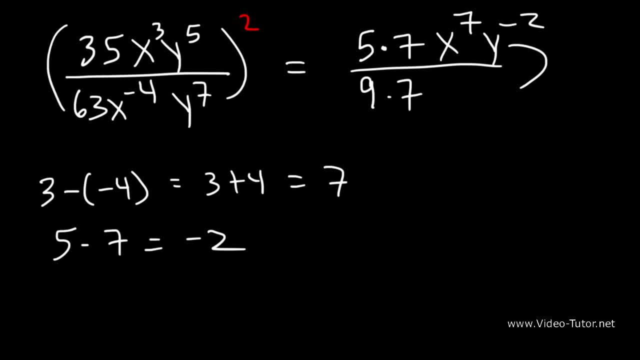 It's negative 2 on top, but if we bring it to the bottom it's going to be positive 2 on the bottom. So let's go ahead and do that. And this is still raised to the second power. Now the last thing we could do is cancel the 7.. 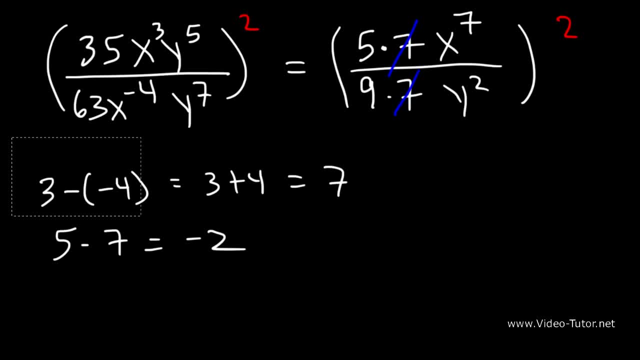 Let's do that again. Let's get rid of this stuff. So we have 5 x to the 7th divided by 9 y squared raised to the second power, 5 squared is 25, and x to the 7th raised to the second power is going to be x to the 14th. 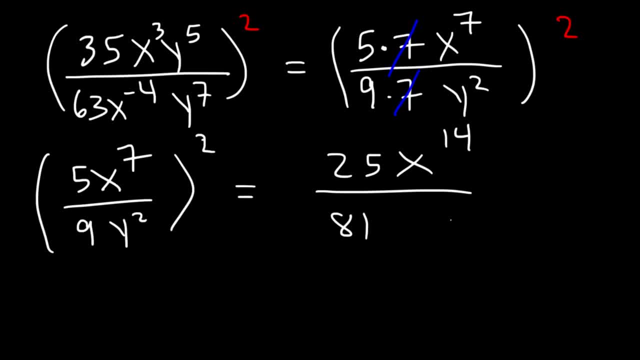 7 times 2 is 14.. 9 squared is 81, and 2 times 2 is 4.. So this should be the final answer.